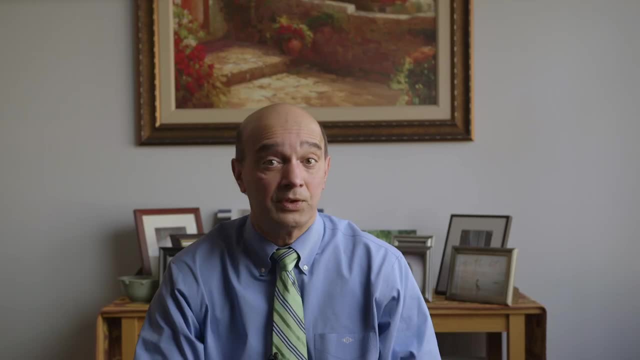 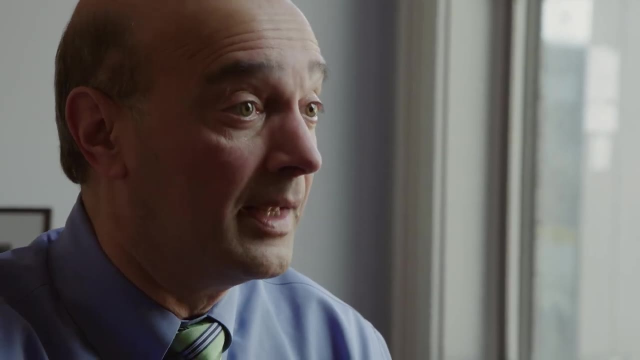 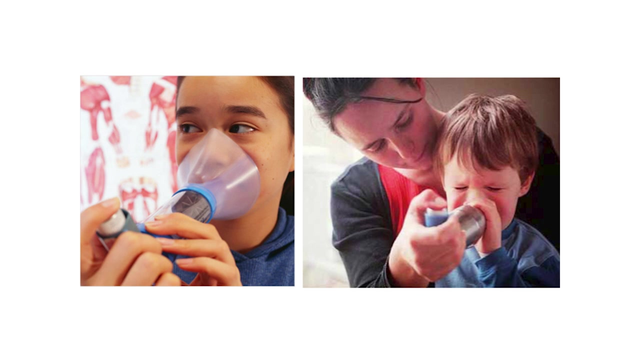 second story is one of a college runner. She was having trouble staying on the team because she was having frequent episodes of wheezing and upper respiratory infections. She has asthma and multiple allergies. She was being treated with inhalers and other medications, but she still couldn't perform. optimally. So more people are on costly medications, and even steroids, to keep their asthma and allergies under control. So we are seeing longer and more intense allergy seasons- from 177 days 10 years ago to 190 days today- and an increase in the levels of air pollution. with 7 million people in the world. living in areas that exceed the World Health Organization limits on particulate matter. More people are seeking care in the office and in the emergency room at a cost of $11 billion per year for allergy care and treatment. So we are seeing longer and more intense allergy seasons: from 177 days 10 years ago to 190. days today and an increase in the levels of air pollution, with 7 million people in the world living in areas that exceed the World Health Organization limits on particulate matter, So more people are seeking care in the office and in the emergency room, at a cost of $11 billion per year for. allergy care and treatment. So more people are seeking care in the office and in the emergency room at a cost of $11 billion per year for asthma care. The third story is a patient of mine who went hiking in Arcadia this summer with some friends. 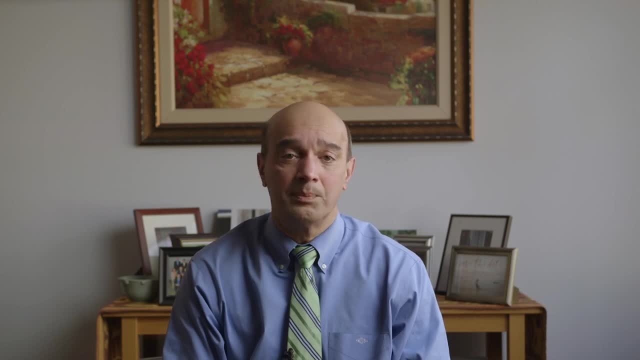 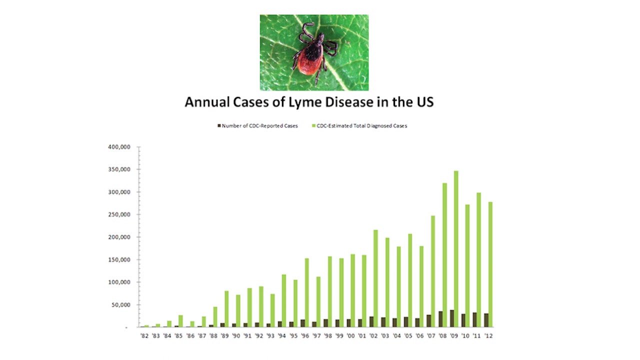 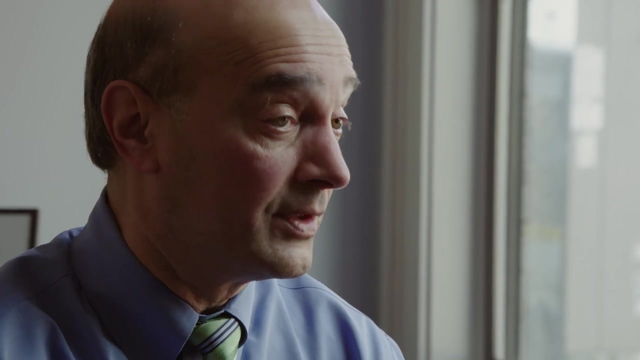 He presented to the office with a rash and joint pains. a few days later He had Lyme disease and Babesiosis. Both are tick-borne illnesses and we've seen a tenfold increase in their incidence in the past several years. In addition, vector-borne illness like Zika and West Nile virus and Eastern equine encephalitis. 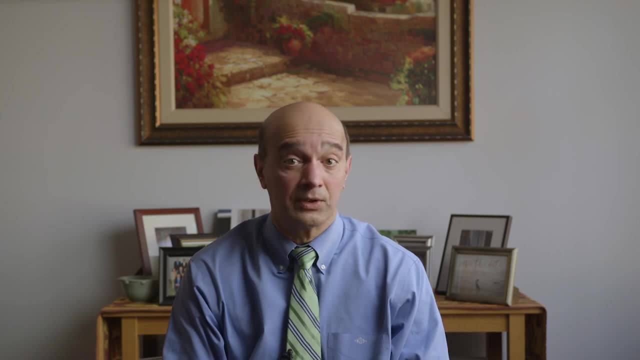 from tick bites, sand flies or mosquitoes is significantly more common and a result of warming temperatures for longer periods around the world. My fourth story is a patient who went to a cilantro bar and about a day later developed diarrhea and abdominal pain. He had a heart attack. 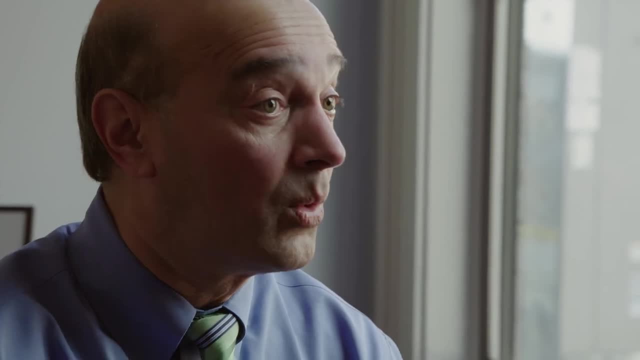 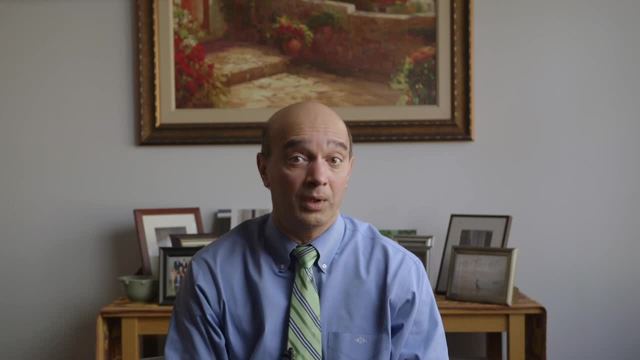 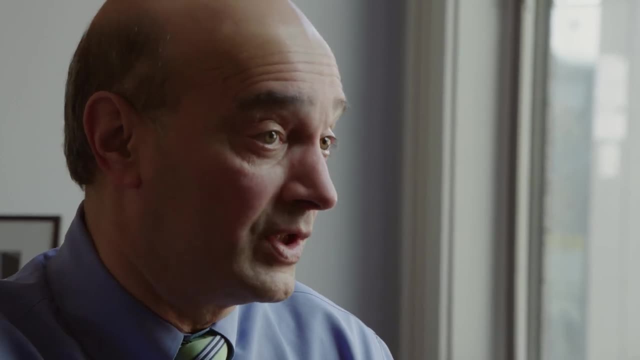 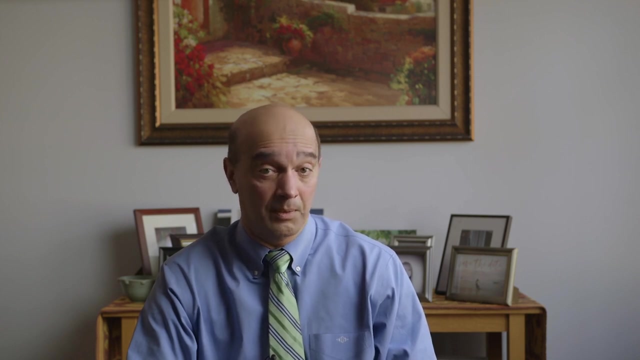 She was healthy, but had acquired a parasitic infection called Giardia from spoiled foods. We are seeing exponential growths in the number of viral, bacterial and parasitic infections from a disruption in food production, shipment and storage from farm to table due to increased 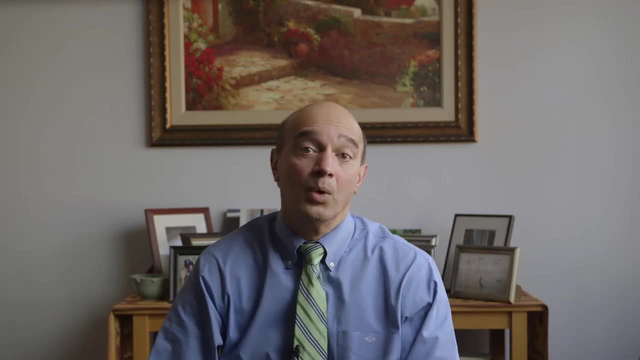 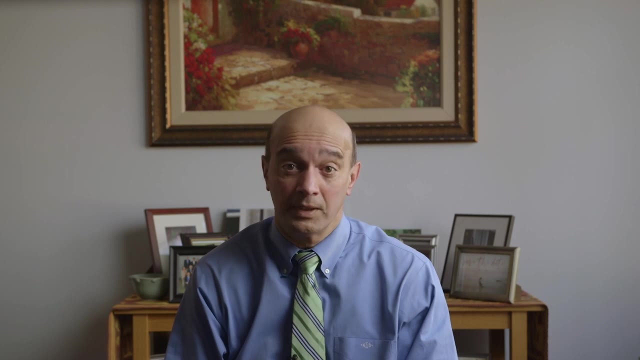 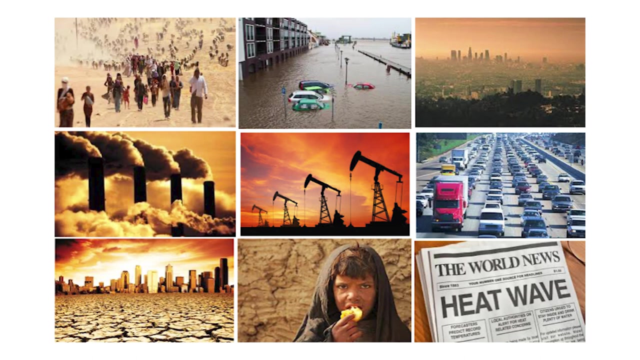 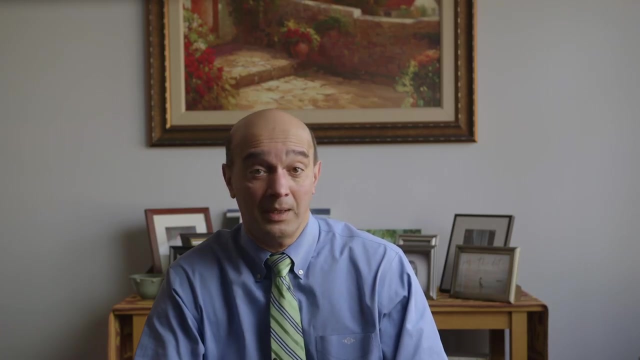 temperature, flooding, extreme weather events- incidents of the four stories I shared with you are exponentially more common today than even a decade ago. In addition, we are seeing more food insecurity, effects on mental health and mass migration around the world. Climate change affects our environment, our health and quality of life. 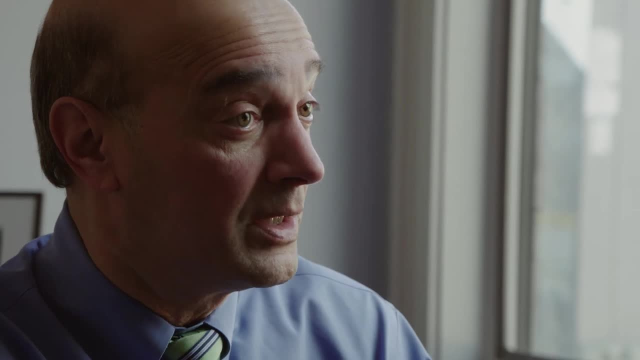 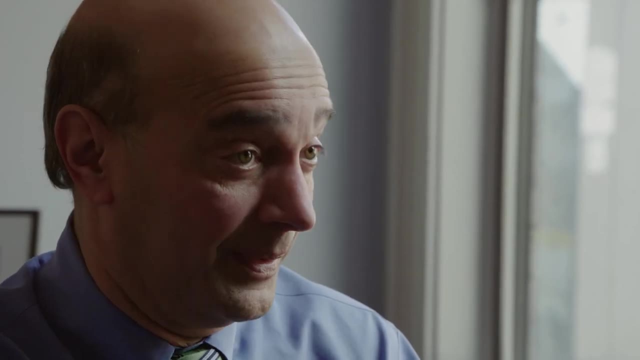 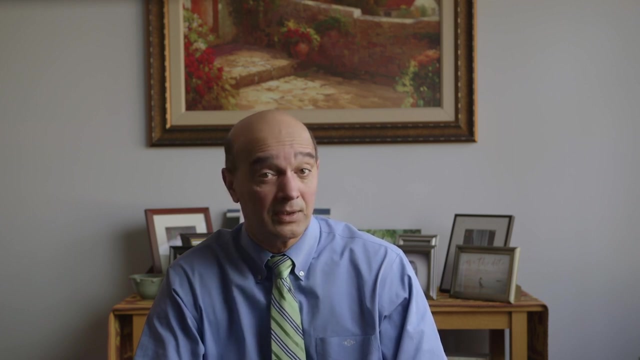 It disproportionately affects our most vulnerable populations: the elderly, the frail, the very young, the poor and communities of color. The warming earth leads to an increase in heat waves, air pollution, melting of arctic ice, sea level rise, increased frequency and intensity of forest. 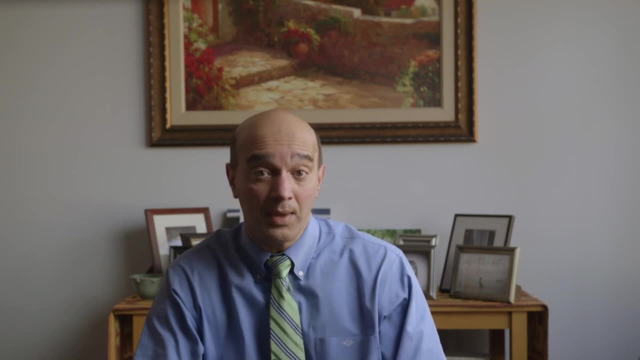 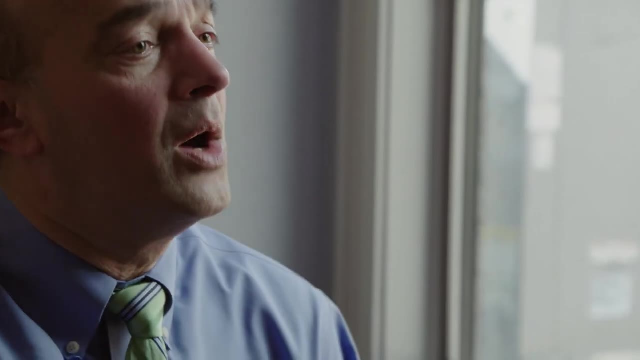 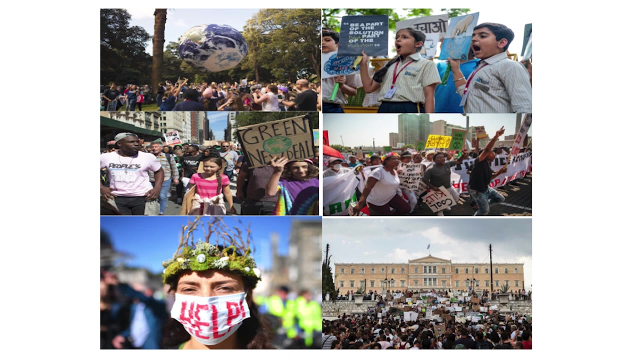 fires, frequent flooding, extreme weather events and mass species extinction. It is not hyperbolic to say that if we don't act now, it will result in an uninhabitable earth before the end of the century. So we have one last opportunity to save the planet and ourselves. 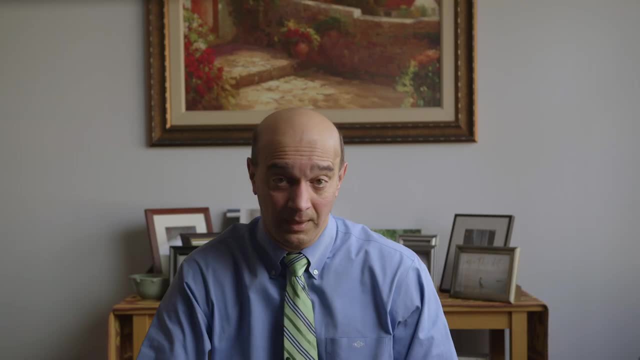 and mitigate the effects of climate change. We need to move to 100% clean renewable energy- that is, wind, solar, hydrogen and safe nuclear- within 20 years. We need to develop sustainable economic and financial incentive through innovation and green jobs. 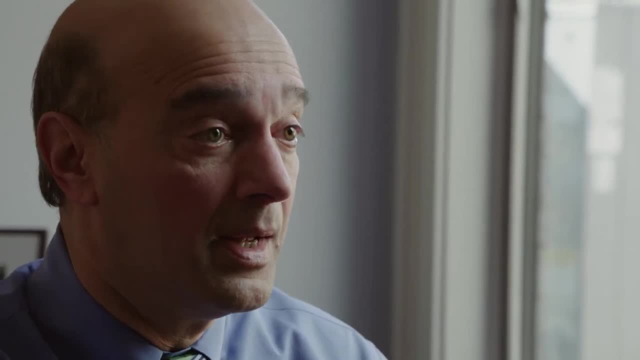 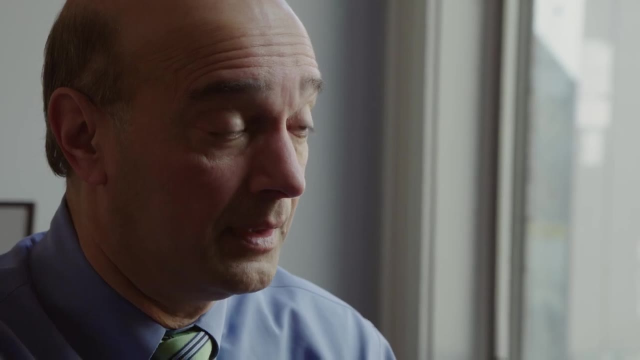 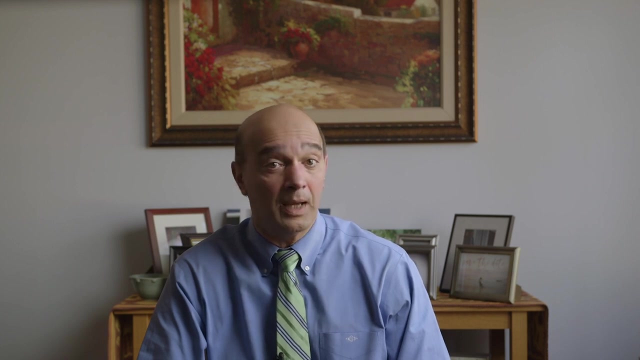 All nations need to commit to this. through the Paris Accord and the upcoming COP26 agreements in November of 2021 in Glasgow, Scotland. You and me, as individuals, can make a difference in mitigating climate change. People are mobilizing all over the world. We need to spread the word. 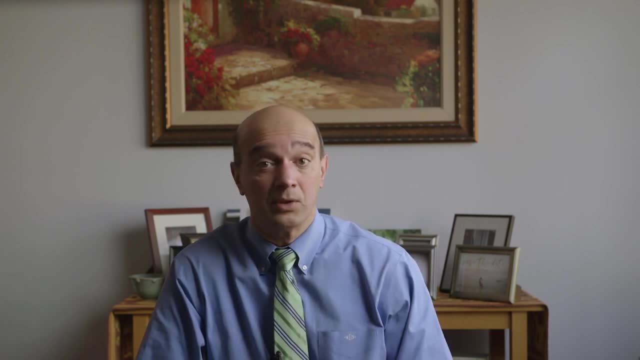 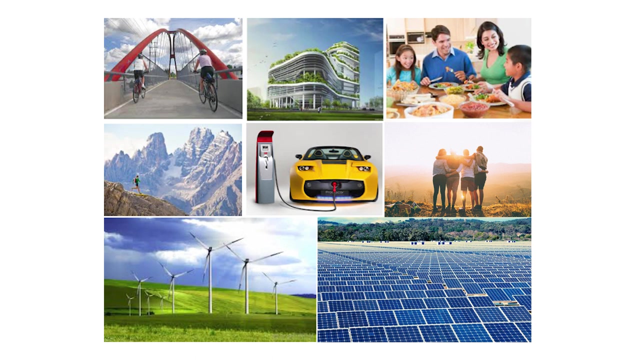 with local, state and national leaders, in your civic organizations, in our schools, colleges and universities About the effects of climate change on our health. We need to eat healthy, plant-based diets, use renewable energy such as electric cars and solar panels. for our homes We need to plant a tree. 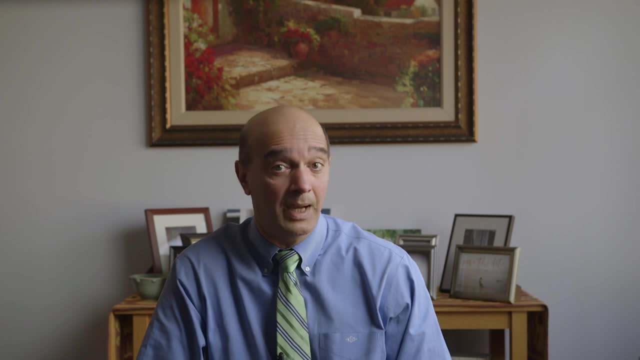 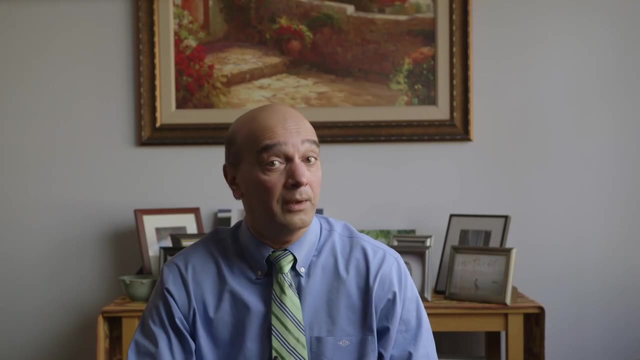 commute less, walk, run and bike and lead healthy lives. So just ask yourself: which world do you want to live in? A world of famine, drought, heat waves, mass migration, violence and air pollution? Or one of healthy diets, biking and hiking?